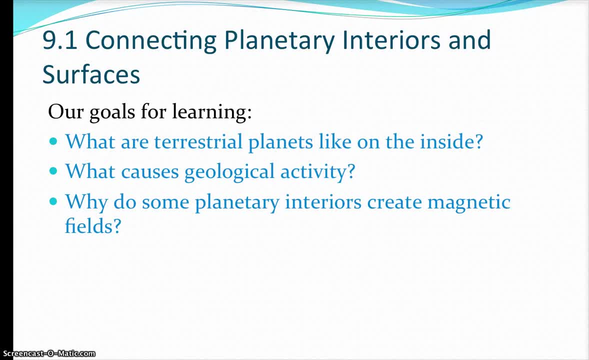 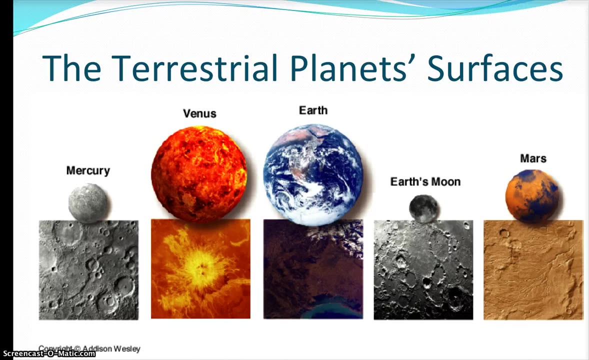 want to learn about is: what are the terrestrial planets like on the inside, what causes their geological activity and why do some planetary interiors allow a planet to create a magnetic field? So first we're just going to start off by looking at these terrestrial planets and what 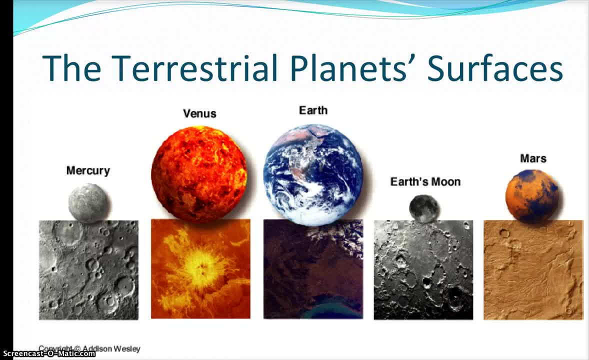 their surfaces look like. Notice, as I said, the moon is pretty similar in size to Mars. It's very similar to Mercury, and so that's why we include it in our study. Also, notice, when you look at the surface of the moon in Mercury, it's very heavily cratered. so they have that in common as well, and we'll 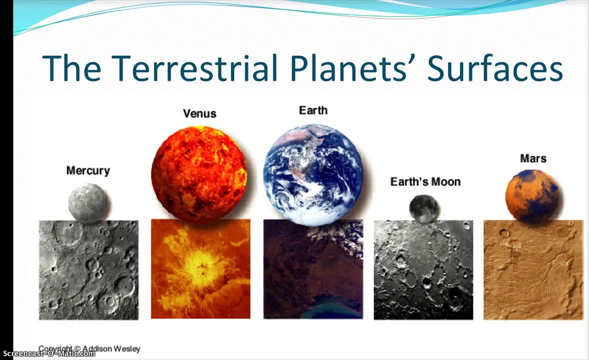 talk about why that might be true. We look at Mars and we see some craters on the surface of Mars, but we also see some signs, like over here, where it looks like there's signs of past water flow, which is one of the reasons that. 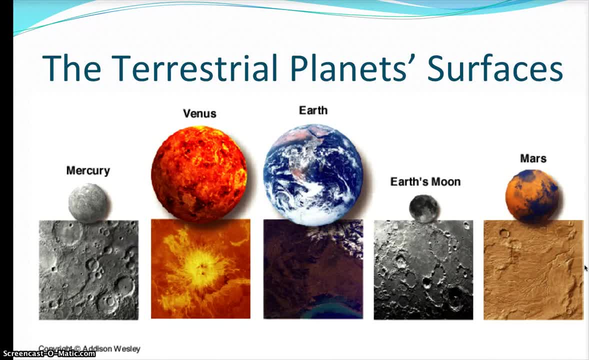 Mars is so interesting to us. When we look at Venus, we actually see a very new surface due to the fact that Venus has had at least very recent, if not present, volcanic activity. And then, of course, the Earth, which we're very familiar with, has a very new surface caused by the 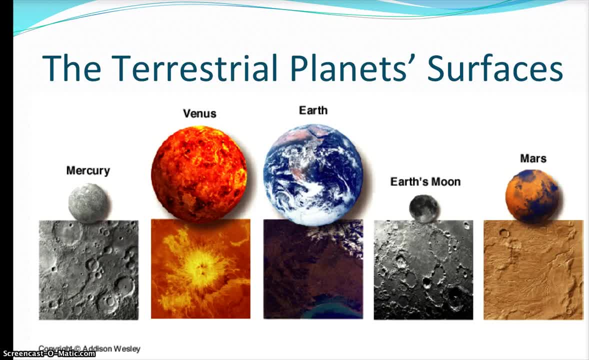 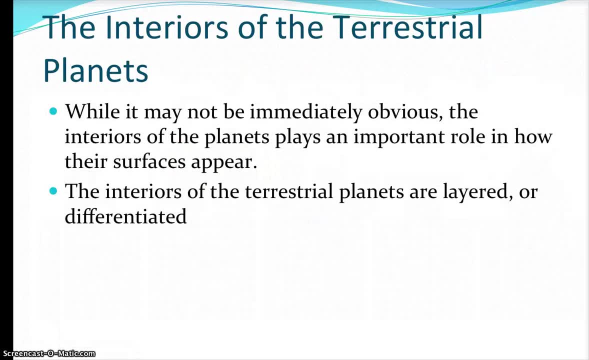 weather, water, wind and all the different planetary processes that cause its surface to be constantly changing. So let's first start thinking about the interiors of the terrestrial planets. We might not really realize this, but the interiors are important because the conditions on the 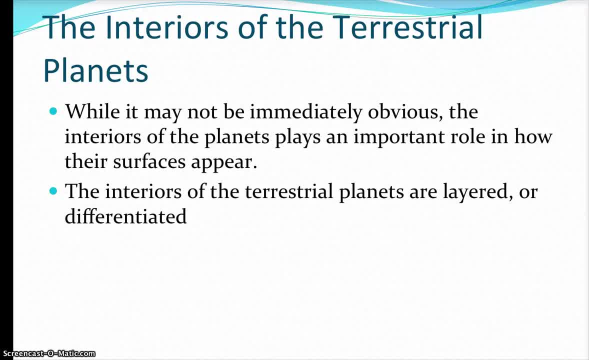 interior of the planet is actually going to play an important role in how their surfaces appear, because it will determine how geologically active and whether the surfaces can change through any sort of interior processes. We're going to see that the interiors of the terrestrial planets are layered or differentiated. Here's a picture of a 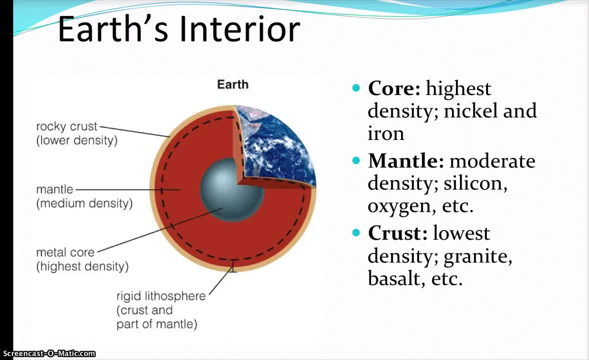 picture of the Earth's interior where we see this differentiation. The three major areas of the Earth's interior are the core, the mantle and the crust. We're starting at the very center with the core, where the highest density material is. 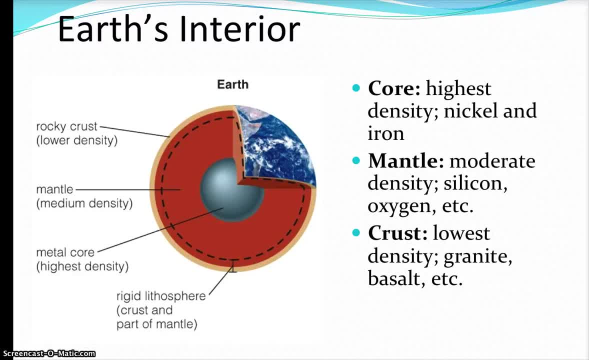 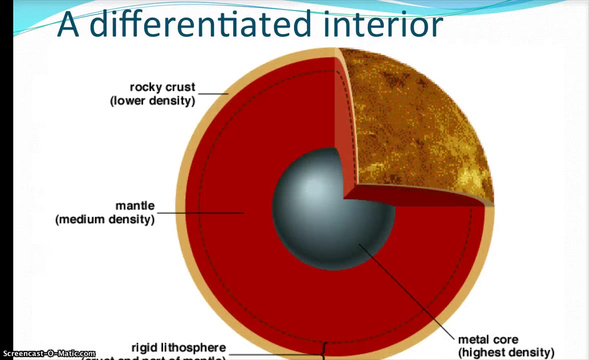 We move on to the intermediate layer, which is the mantle, which has an intermediate density, And then, finally, at the surface, we have the crust, which has the material of the lowest density. This is what we mean by differentiation: is that the interior has separated into different layers of different densities. 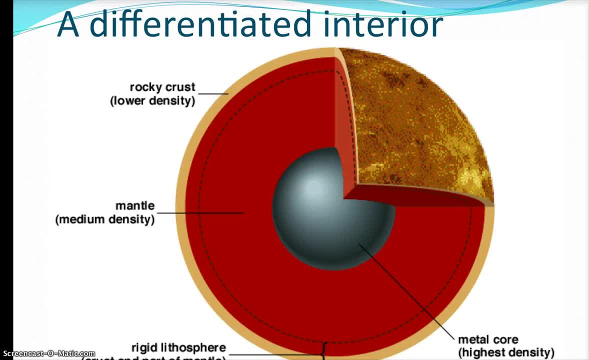 Here's just a more general interior showing the differentiation. Another thing that we will be looking at in some of the planets is this area here that is a portion of the crust and the upper portion of the mantle, which we call the lithosphere. How much of the planet's interior is included in the lithosphere has a lot of plays a large role in determining how geologically active that planet would actually be. 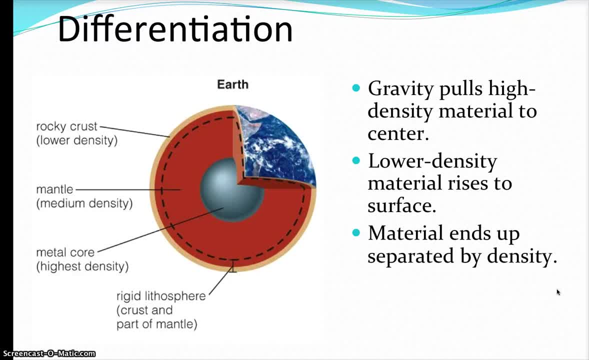 So, as I said, the differentiation is the different layers of different density, And the reason for this is that gravity has pulled the higher density material to the center and then the lower density material has rise to the surface. An analogy I like to think about is if we took a handful of dirt, rocks and leaves and threw them in the water. 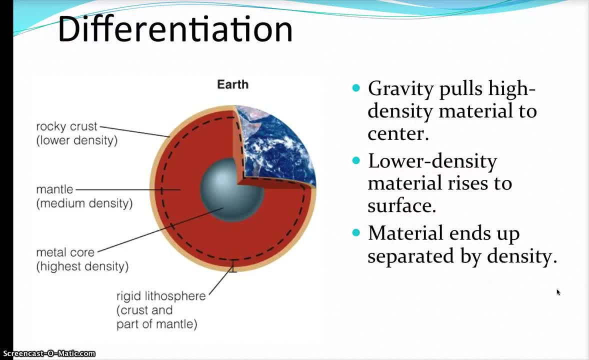 The rocks would sink immediately to the bottom of the water, while the dirt would sort of percolate down or drift slowly down, while the leaves would float on the top. This is sort of a simulation of what I visualize when I think of the differentiation of the interiors of the planets. 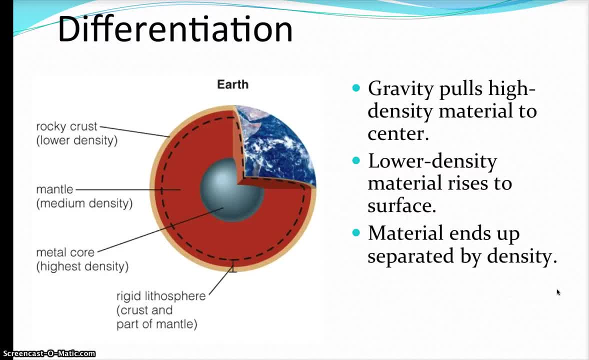 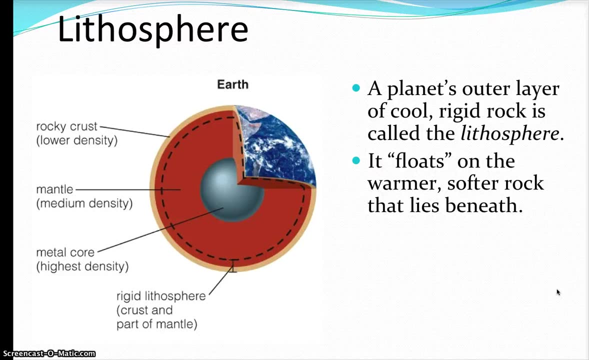 It's just in one dimension instead of the three dimensions. So the heavier materials sink to the very center of the planet and then, as we move our way out, we have lower density material. As I also said, we want to be familiar with the lithosphere, which is the outer layer of cool, rigid rock. 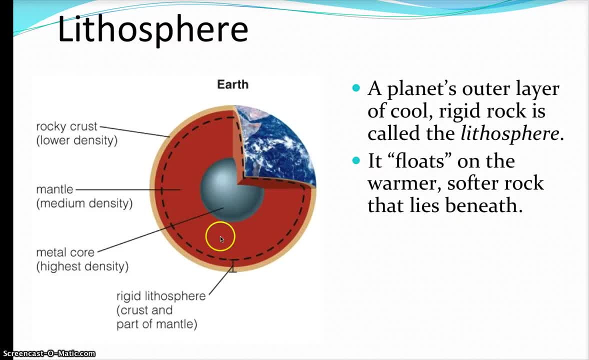 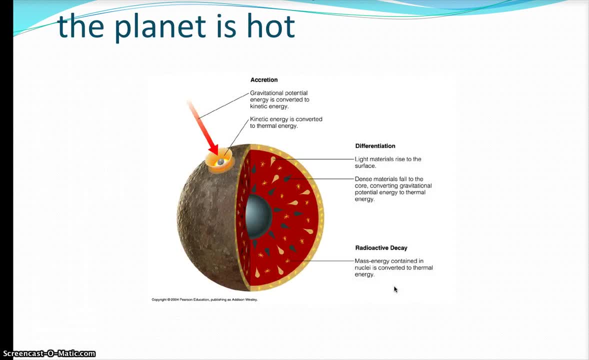 And it's actually sitting on the mantle, which is a warmer, softer rock that lies underneath it. The differentiation, we believe, is the temperature. The lithosphere, we believe happened early in the planet's history, when the planet was still warm. 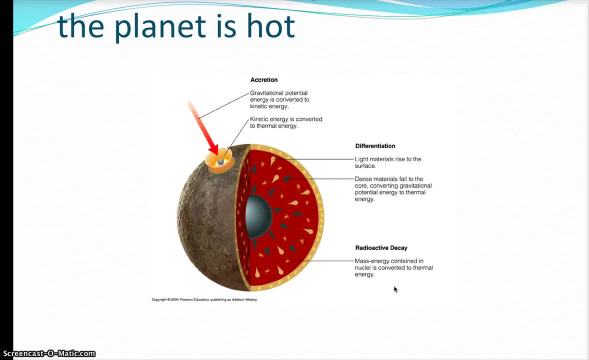 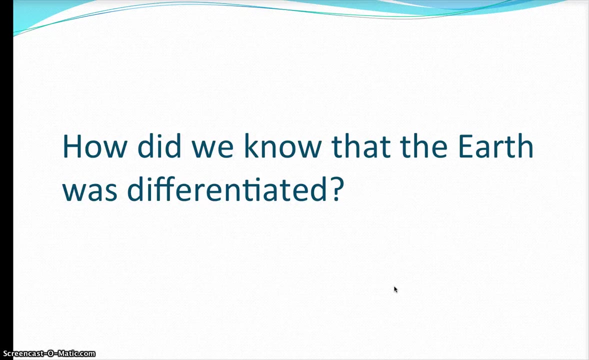 and the material was in a molten state so that it was able to move, And that's when the heavier material sank to the center of the planet, leaving the lighter materials at different areas. So you might wonder how we know that the Earth is differentiated. 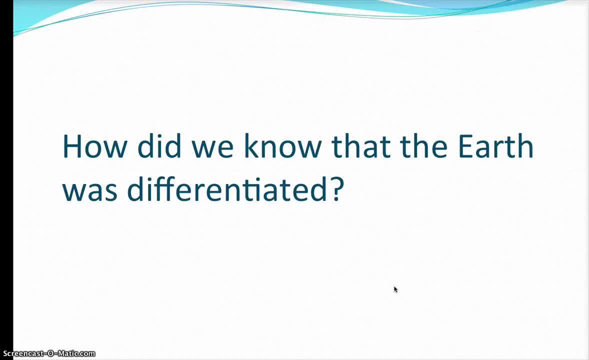 At first you might think: well, we probably just have drilled down into the core of the Earth and that's how we figured it out. But we haven't. We haven't actually even penetrated the crust of the Earth with our drills, So we have to sort of learn indirectly. 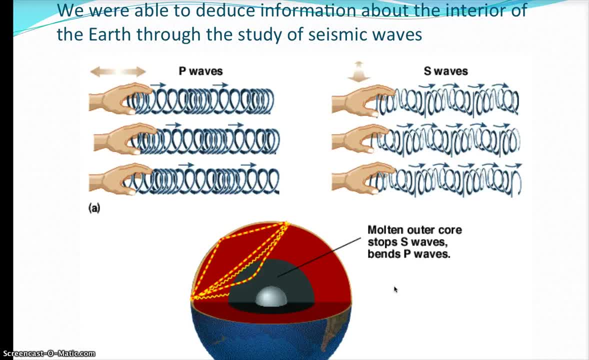 And the way that we learn is through seismic waves. Those are the waves that are created during an earthquake. There are two different types of seismic waves. The first is called P waves or pressure waves, And these are the kind of waves you would produce if you took a spring and you moved it fast in and out. at the end, 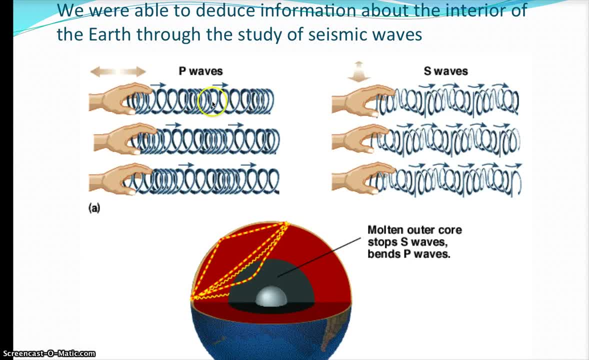 They create areas where the spring is compressed and other areas where the spring is spread out, And those areas spread through the spring as they travel. The S waves are another type of wave that were probably the type of wave that we're more apt to visualize when we think of waves. 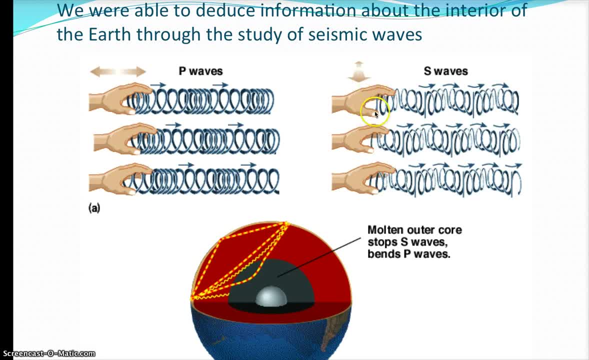 The S waves, or shear waves, would be caused if we would shake the spring up and down. So what happens when there is an earthquake? Both types of these waves are created And they travel through the interior of the Earth. It turns out that S waves cannot travel through liquids. 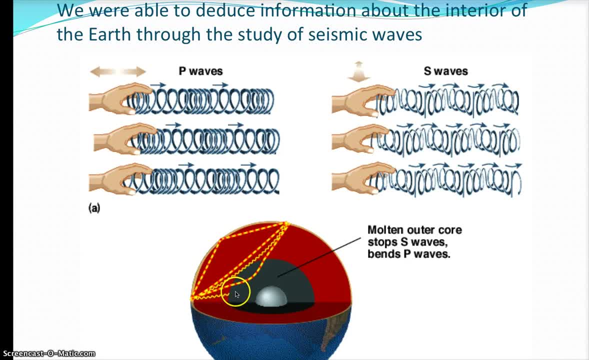 So we know that the S waves have hit some sort of liquid part, because the outer part of the core is actually liquid. So we've been able to figure that out by the absence of the S waves at some other monitoring station. So if the earthquake was here and we were monitoring here, 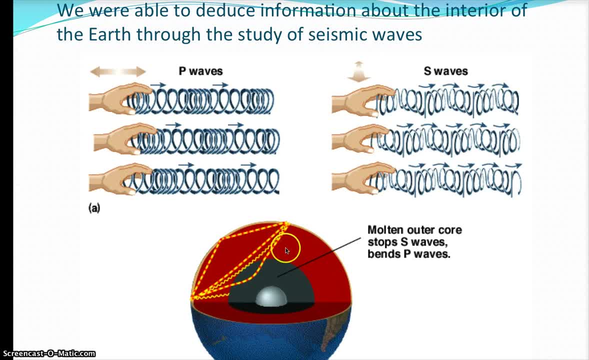 we would see that this S wave was there And this S wave never actually got to this point. The other way that we can learn more about the interior through these waves is the fact that the speed of the wave travel will depend on the density of the material that it travels through. 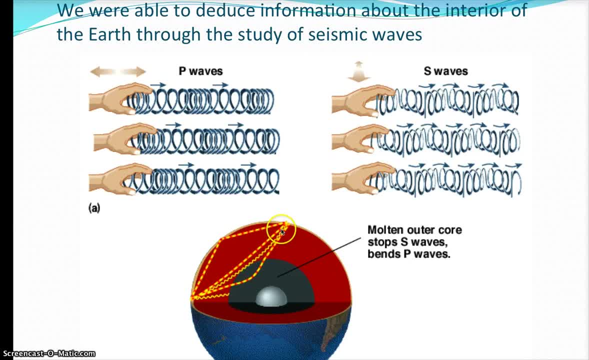 So from that, by the amount of time that it takes the different waves to arrive at a particular location, we're able to calculate what the density of the material that the wave actually would have traveled through. So it's actually a lot more complicated than what we thought. 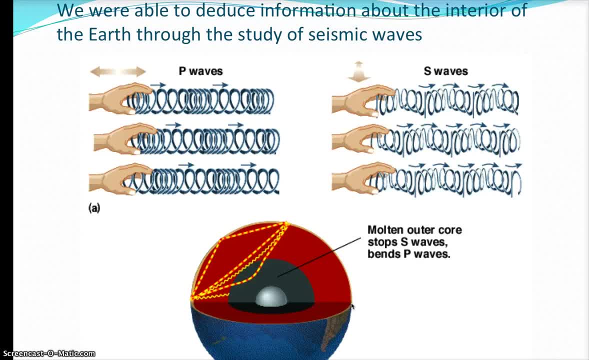 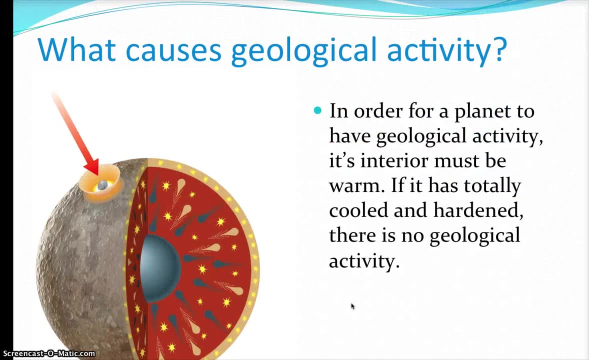 To be able to calculate the density of the material we would have to go through different waves. very interesting how we've been able to use earthquakes to study the interior of the earth and gain information about the interior without actually ever going down and physically seeing what's going on. so when we talk about a planet, we're 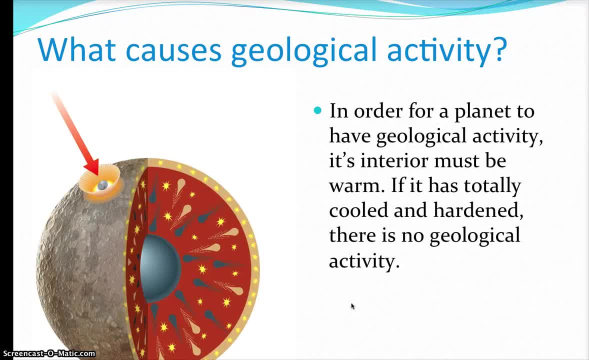 interested in geological activity, because this is how the surface, one of the ways in which the surface can be changed is through volcanic activity or tectonic plate movement, and so this, those kinds of things, can only happen if the interior of the planet is warm, if the planet has cooled off and the rock 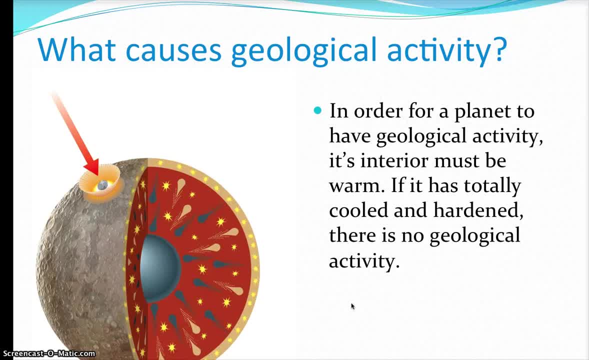 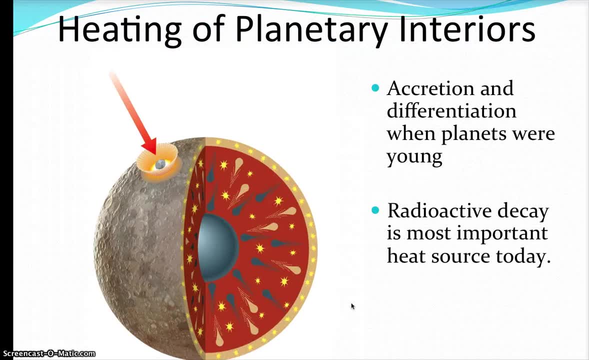 has hardened, then nothing's happening inside of the planet and geological activity such as volcanism is not going to be occurring. the heat that we are thinking about. why would the planet be warm? well, the planet is warm from the time then it was formed, as it was compressed and the accretion took. 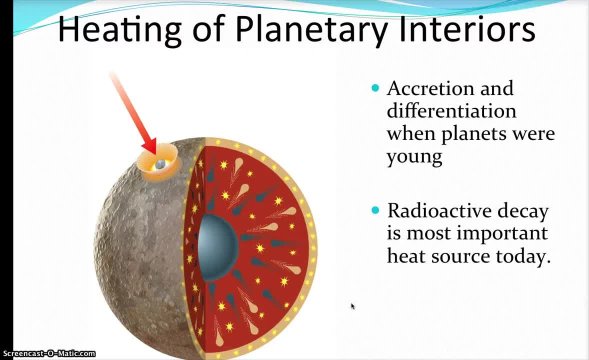 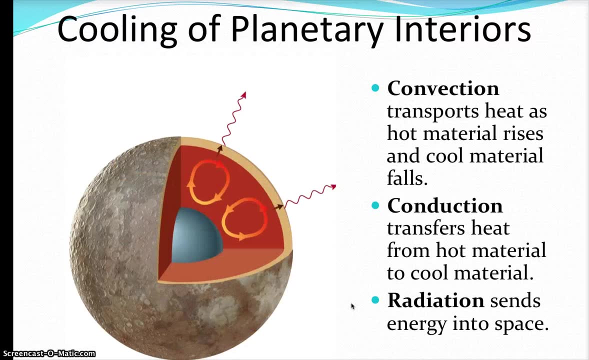 place. that caused some heat to be sort of stored within the planet. the other thing that happened is the radioactive decay that occurs within the interior of the planet also helps to heat up its interior as time goes on. this heat is given off by the planet, and as it gives off, 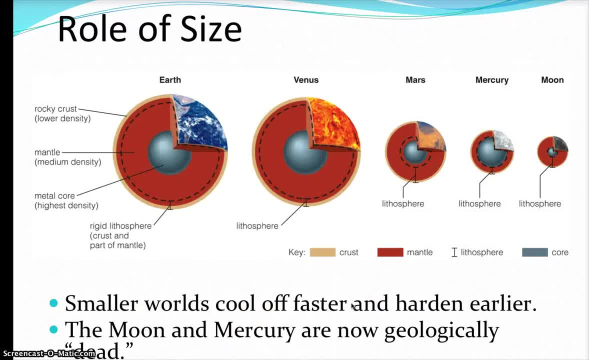 that heat, it begins to cool. so what we find is that the size of the planet is going to play a very important role in how cool, how much it has cooled off since it's been formed and then, of course, following that, how geologically active it is. so here now we're going to focus on that thing called the.